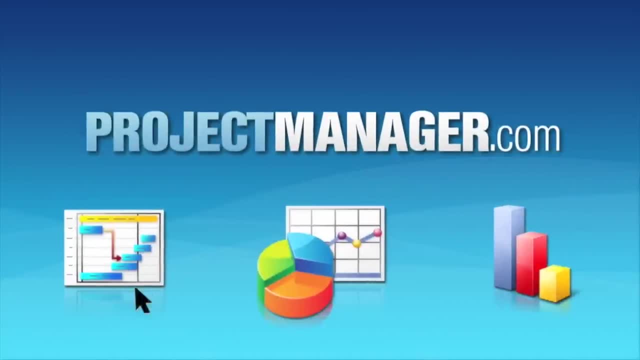 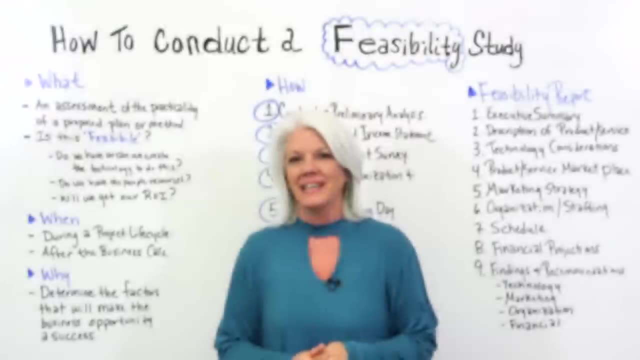 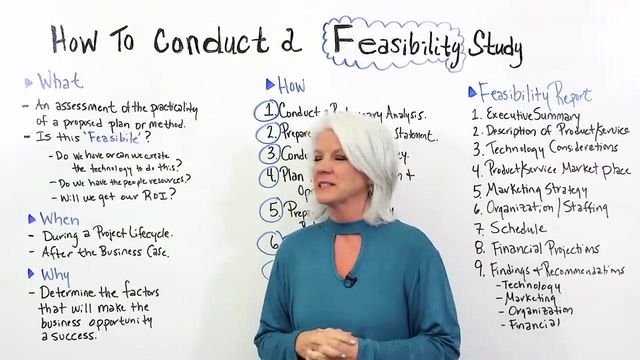 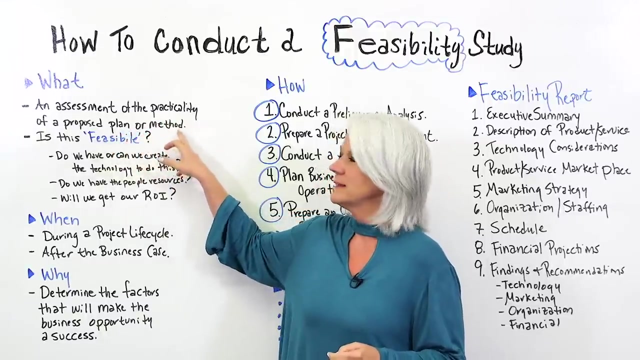 Today we're talking about how to conduct a feasibility study, But first of all I want to start with clarifying what a feasibility study is. Basically, it's an assessment of the practicality of a proposed plan or method. Basically, we want to know: is this feasible? 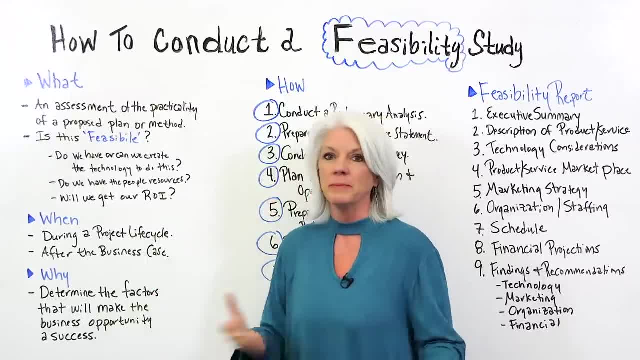 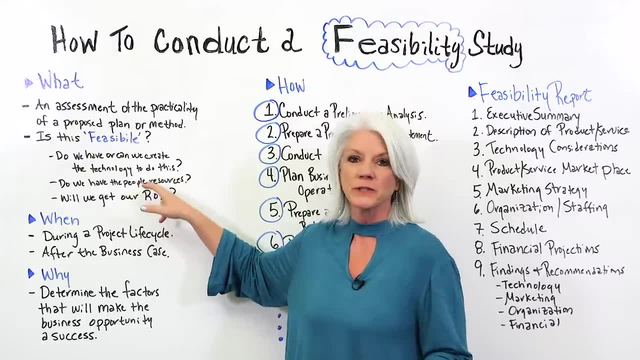 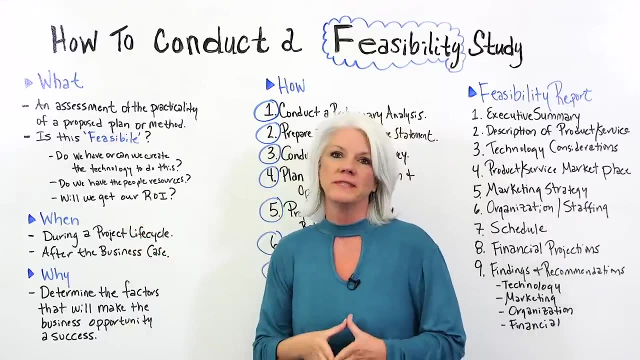 Some of the questions that may generate this, or we can hear people asking, are: do we have or can we create the technology to do this? Do we have the people resource who can produce this, and will we get our ROI, our return on investment? So when do we do the feasibility? 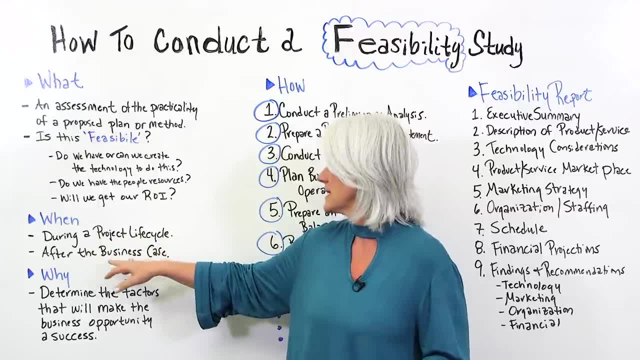 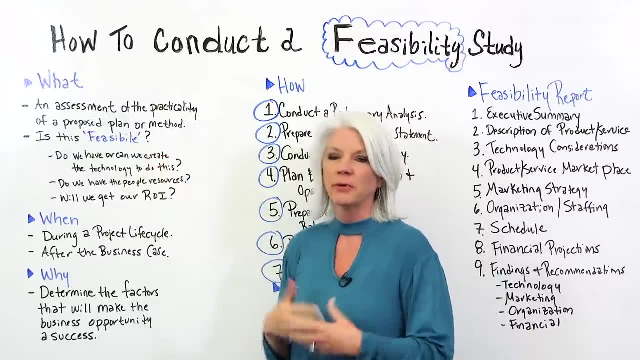 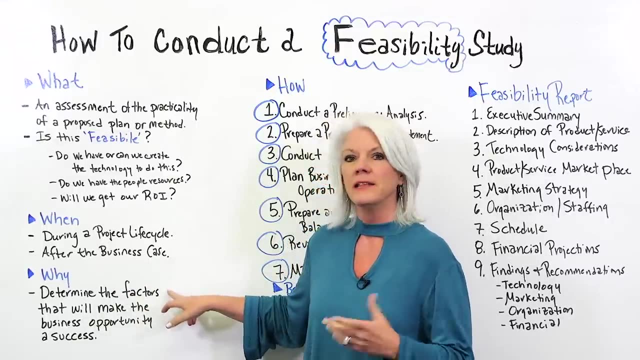 study. So it's done during a project life cycle and it's done after the business case, because the business case outlines what we're proposing. Is it a product or service that we're proposing? So why do we do this? The reason we do this is because we need to determine. 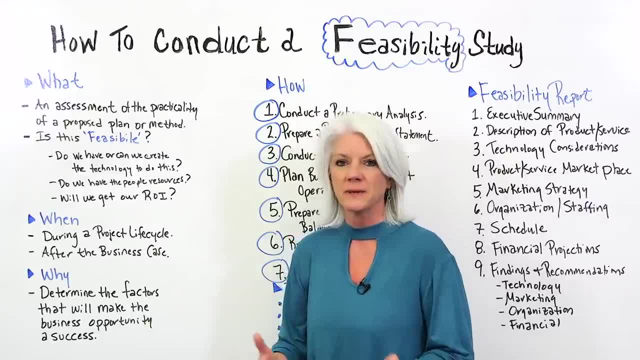 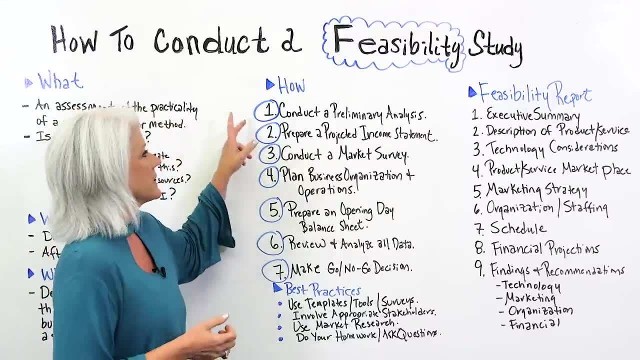 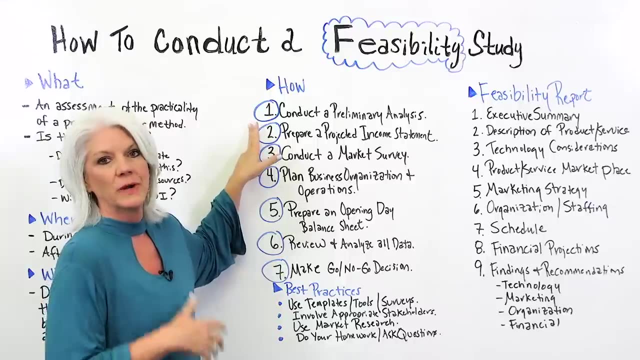 the factors that will make the business opportunity a success. Well, let's talk about a few steps that we do in order to conduct the feasibility study. Well, first of all, we conduct a preliminary analysis of what all is involved in the business case and what we're analyzing and what we're 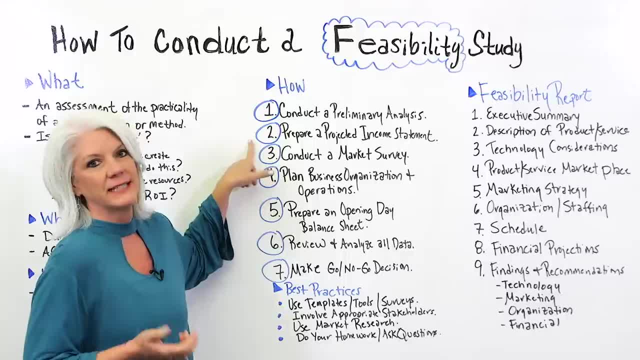 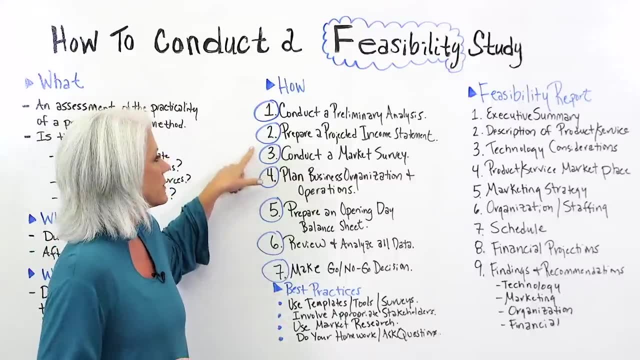 trying to determine is feasible. Then we prepare a projected income statement. We need to know what are the income streams. How are we going to make money on this? Where is the revenue coming from? We also need to conduct a market survey. We need to know: is this a demand? 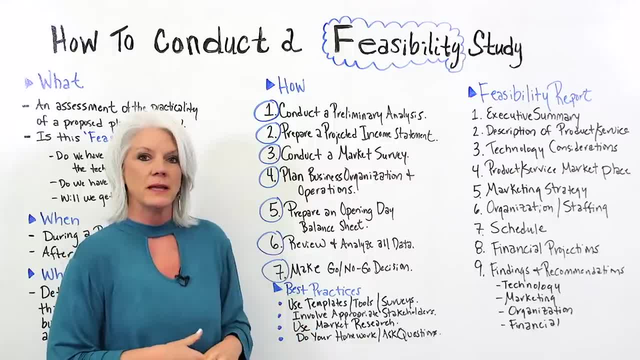 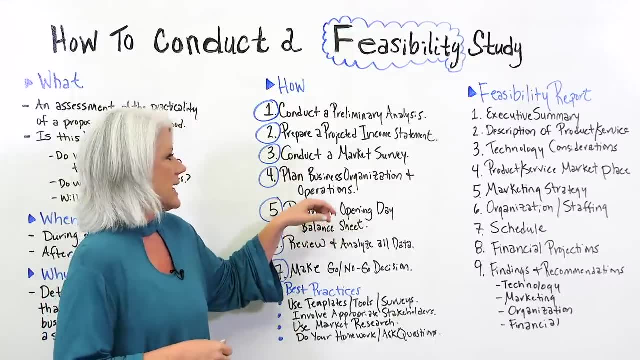 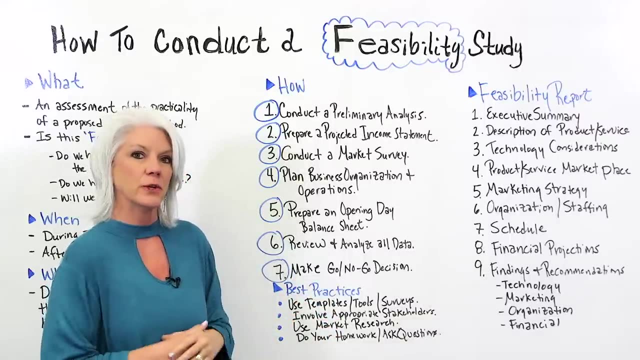 Is there a market for this? Are customers willing to use this product or use this service? The fourth one is: plan a business, the business organization and the operations Like. what is the structure? What kind of resources do we need? What kind of staffing requirements? 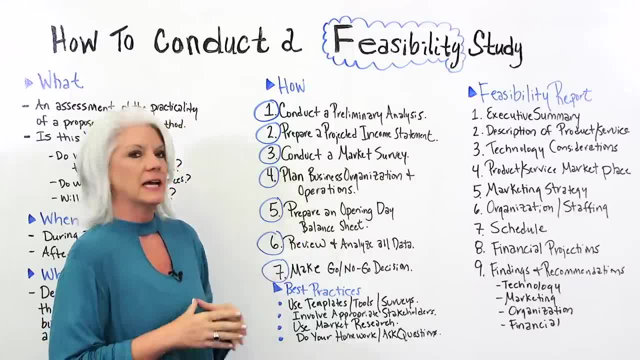 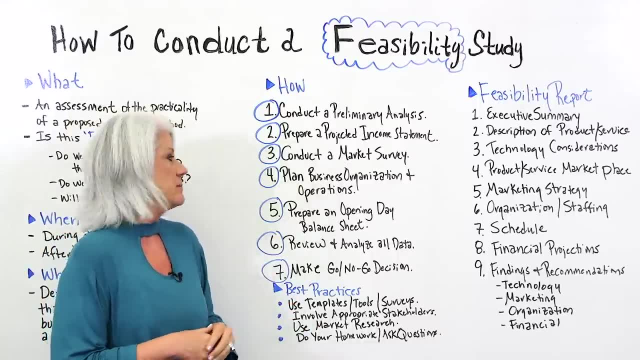 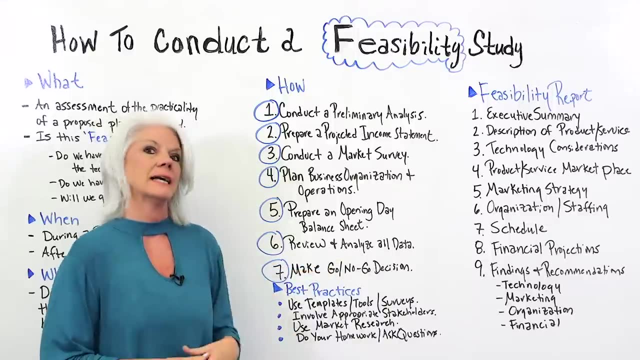 Do we have? We also want to prepare an opening day balance sheet. What are the how? again, what are the expenses, What's the revenue, And, to ensure that, being able to determine if we're going to make our ROI. So we want to review and analyze all of the data that 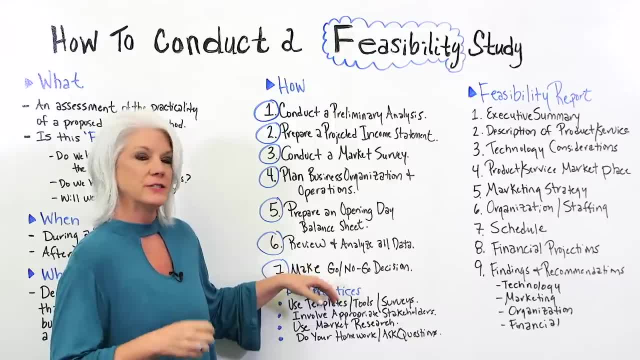 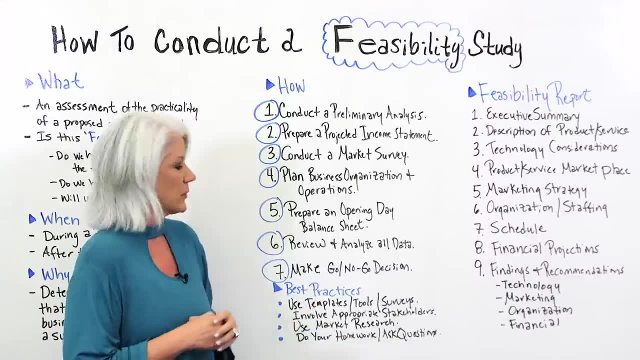 we have And with that we're going to determine- we're going to make a go no go decision, meaning, are we going to do this project or this business opportunity or not? Well, here are some of the best practices to use during your feasibility study. One: 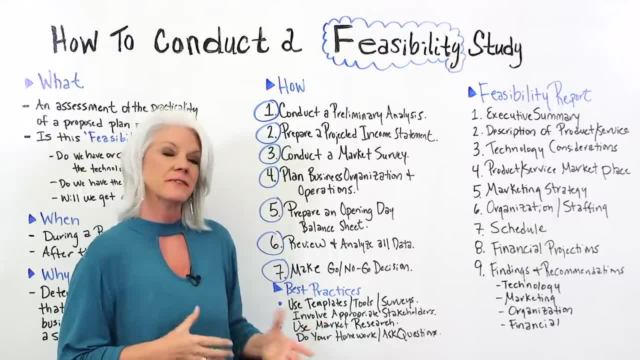 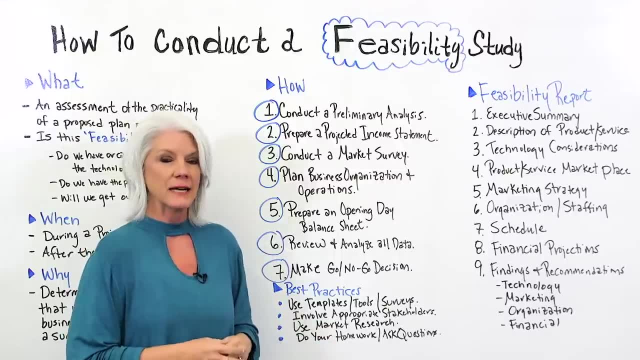 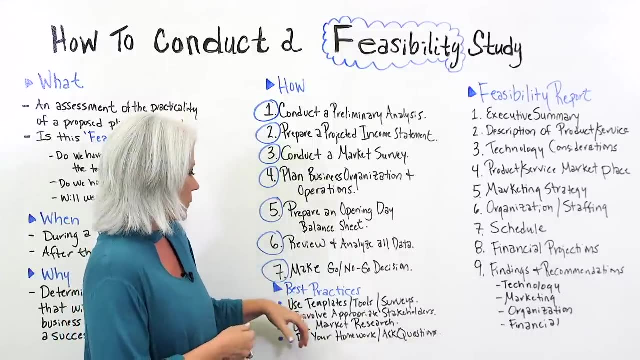 is: use templates, tools and surveys that exist today. The great news is, data is becoming more and more prevalent. There are all kinds of technologies, There are groups that they do nothing but research- Things that we can leverage today. We want to involve the appropriate 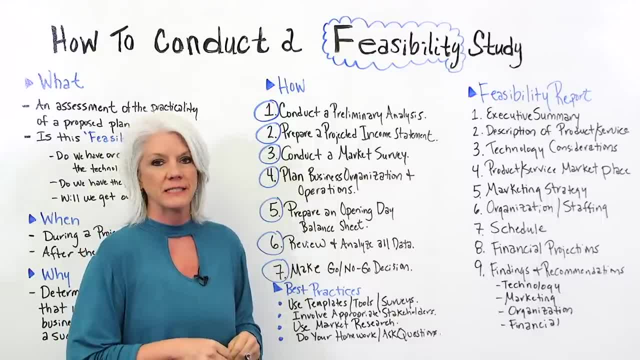 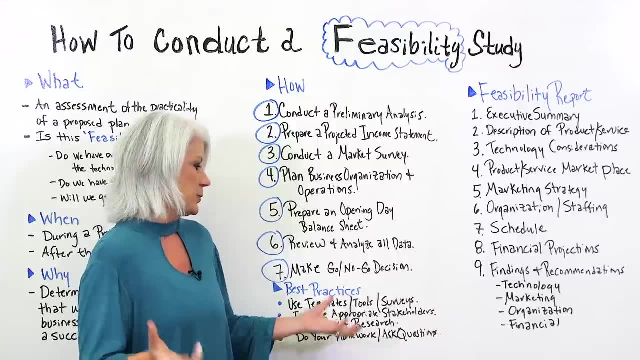 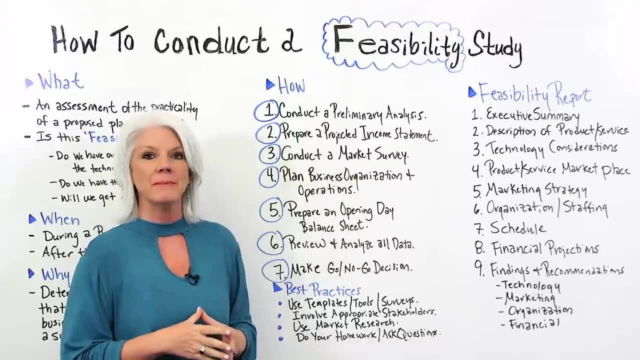 stakeholders to ensure that input is being considered from the different branches of government, from different people involved. We also want to use again the market research to ensure we're bringing in good, reliable data. We also- I mean, do your homework meaning. 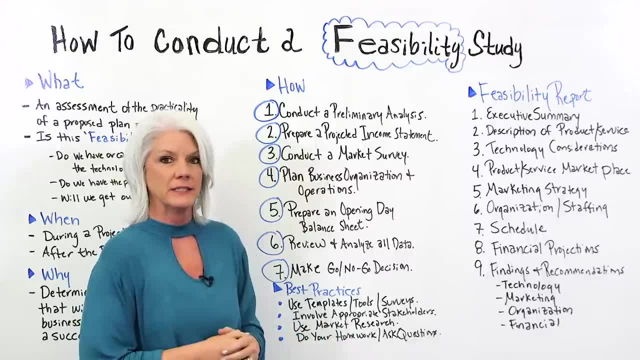 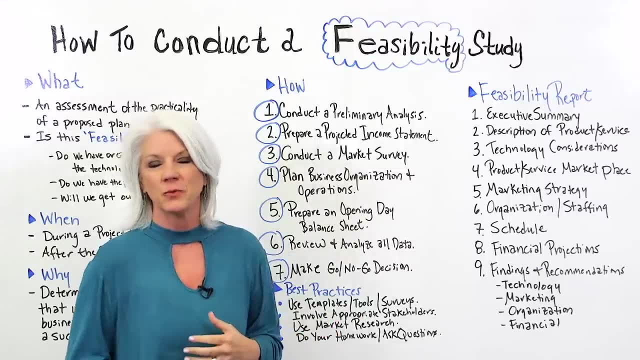 act like as if this is your project, if it's your money, So do your homework and do it well and make sure you give credible data. So, ultimately, in the end, what we're doing is for producing and we're providing a feasibility report. So in that report, this, the feasibility report- will be reviewed. What that report will do. it'll usually be a 360 degree view and then we can provide more information about all of those factors that you guys are making. So if you're interested in going through that data, you can go to the community. go to the community and then we'll. 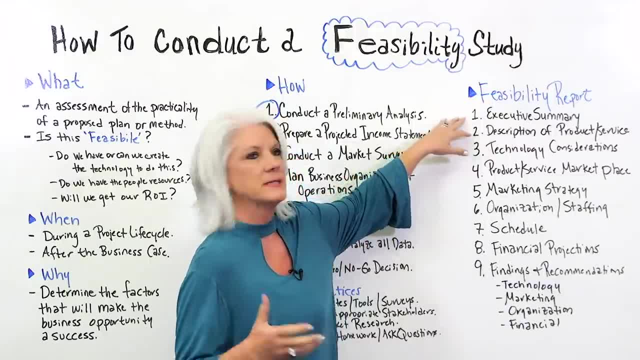 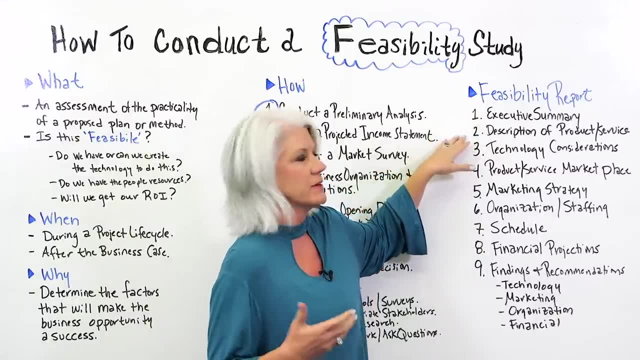 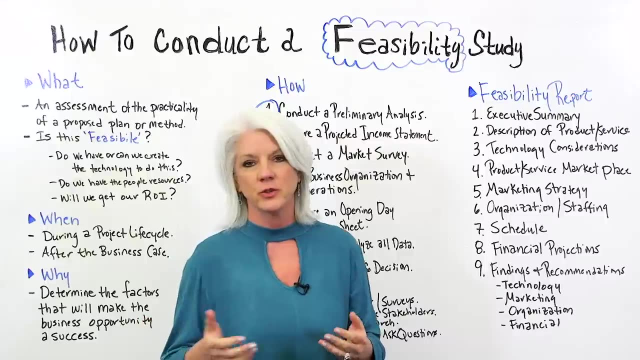 think of this as like a template. So what you're going to do is give an executive summary of the business opportunity that you're evaluating and the description of the product or the service. You want to look at different technology considerations. Is it technology that you're? 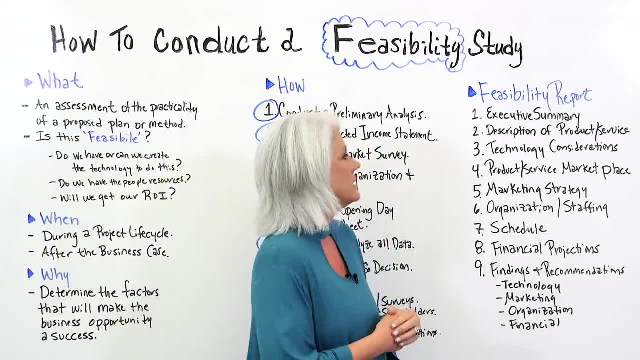 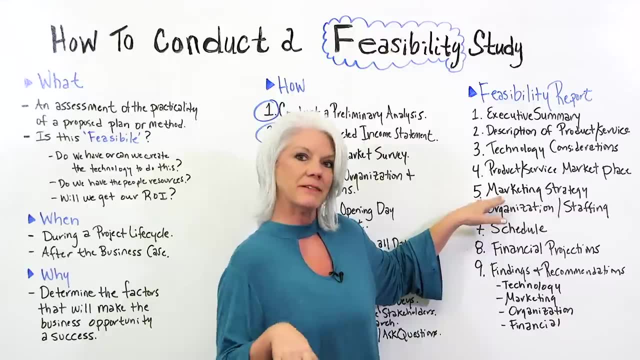 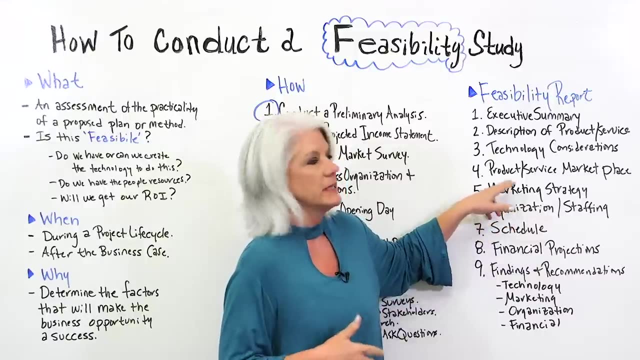 going to use? Are you going to build the technology, What kind of product and service marketplace And being able again to identify the specific market you're going to be targeting? Also, what is the marketing strategy you're going to use to target the marketplace And also what? 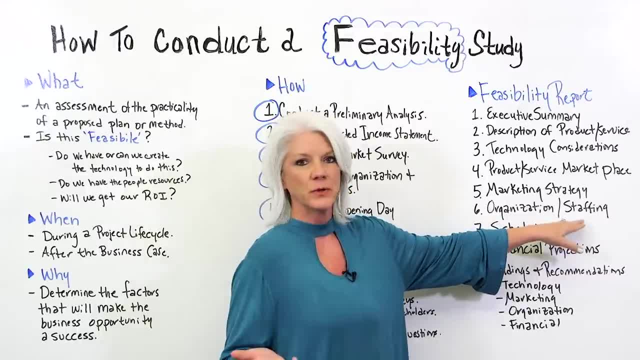 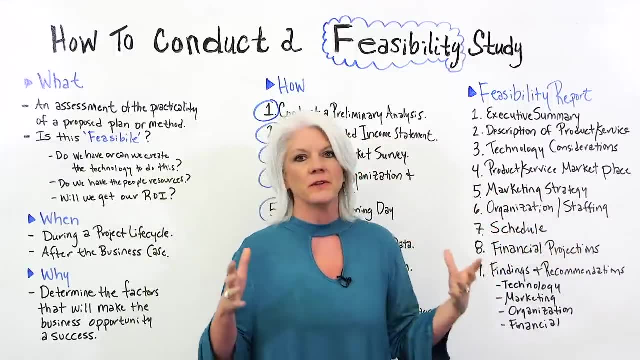 are the? what's the organizational structure? What are the staffing requirements? What people do you need to deliver the product or service and even support it? So also, we want to know the schedule, to be able to have the milestones to ensure that, as we're.